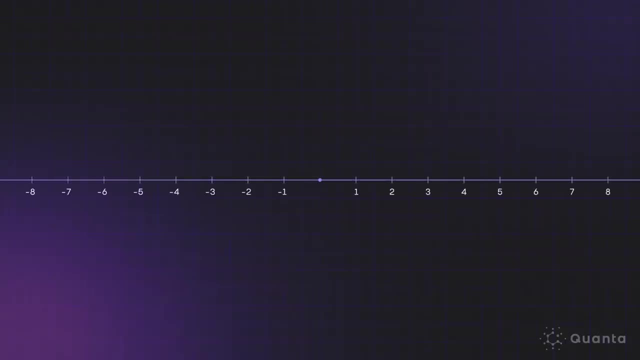 A complex number is defined as the sum of two components: a real part and an imaginary part. Each complex number can be visualized as a point in a 2D plane. The real part is a number found on the number line. The imaginary part is a multiple of the square root of negative one. 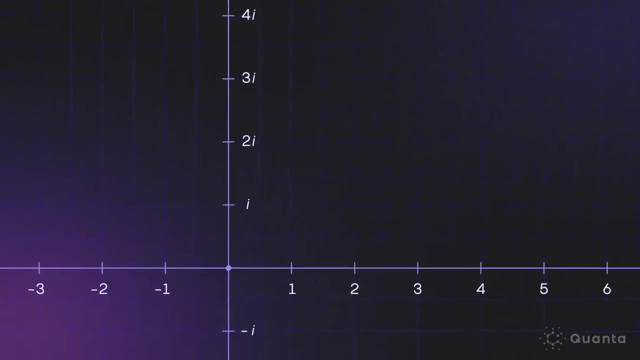 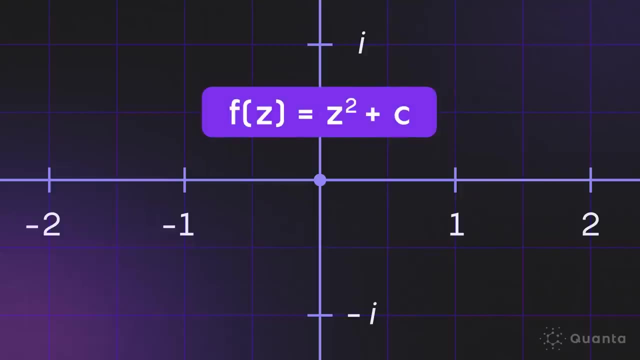 which mathematicians write as i. Despite the name, imaginary numbers play a vital role in solving real world problems. To construct a Julia set, start with the simple quadratic equation: F of z equals z squared plus c. Add a value for c, like negative one, for example. 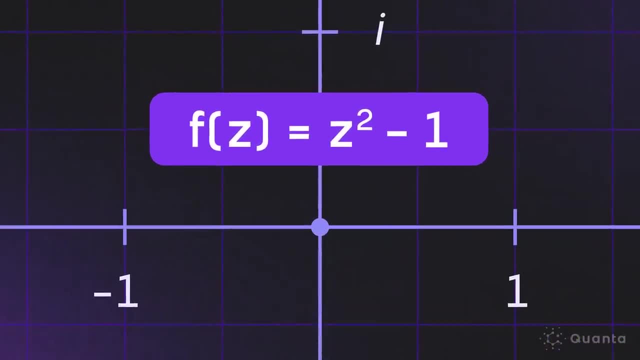 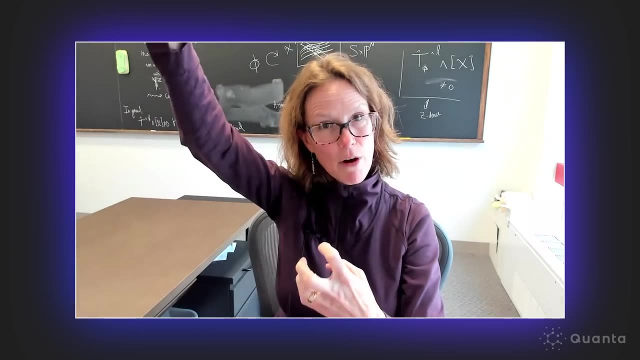 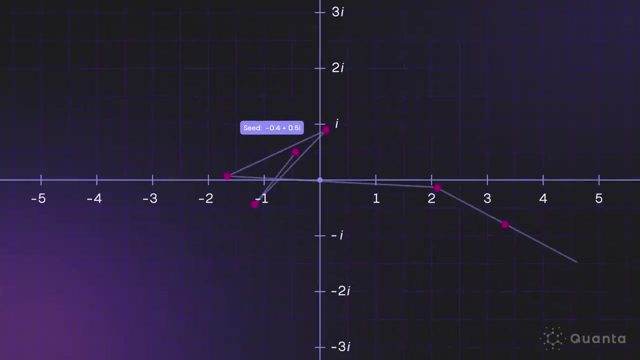 Then consider what happens when you iterate this equation for every possible starting value. You repeatedly apply the function to this sequence of numbers that you're generating and you ask whether or not that sequence is going off to infinity or whether it stays bounded For some initial values. your equation speeds off to infinity when iterated like this. 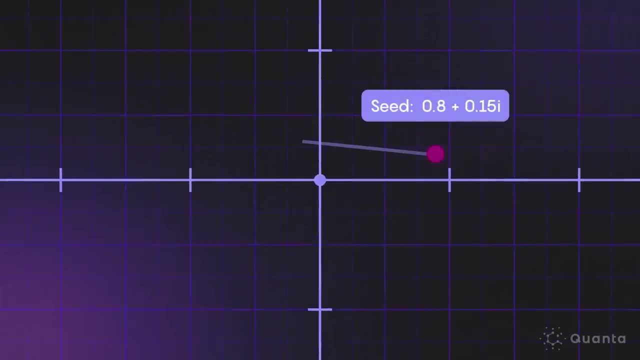 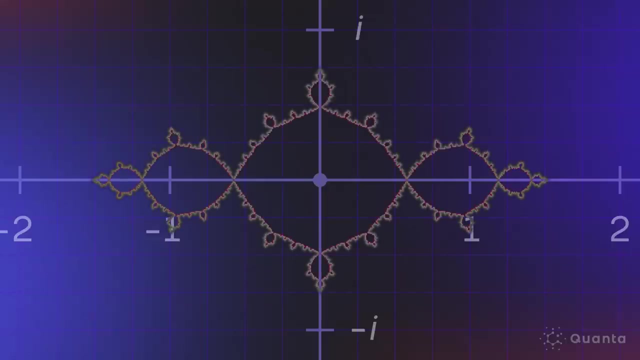 These values are not in a Julia set. When you start iterating from other initial values, you instead get a sequence of outputs that stay bounded When something comes back to itself. often we call that recurrent behavior, and that's where the complexity arises. The boundary between points that stay bounded and those that don't is a Julia set. 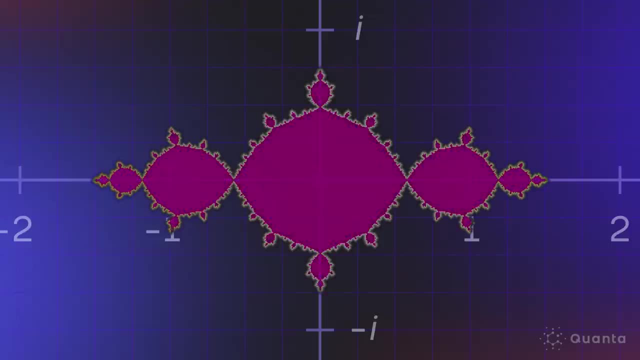 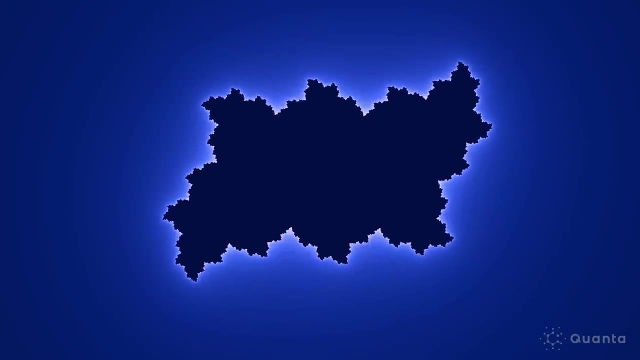 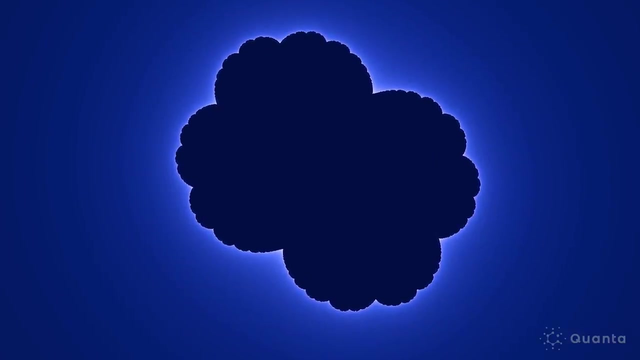 You can fill it in by including all the bounded values. Different quadratic equations generate a wide range of filled Julia sets, from basic blobs to intricate twisting tendrils. Filled Julia sets can be divided into two categories. Sets where you can draw a line from one point to any other without lifting your pen are connected. 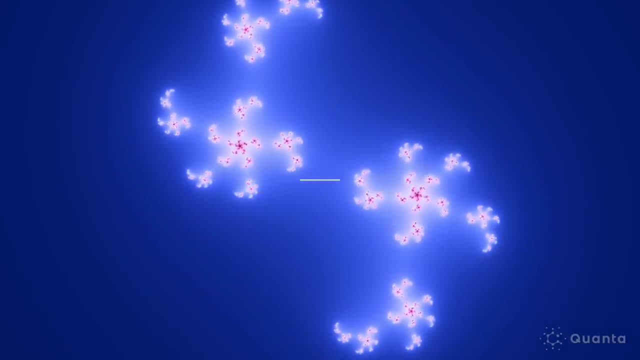 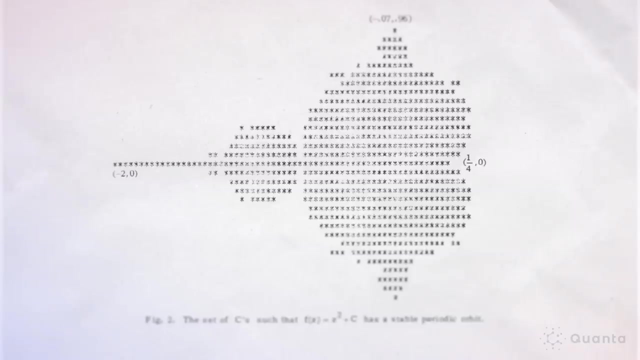 Sets where points look like scattered pieces of dust are disconnected. The first rough plot of the Mandelbrot set appeared in a 1978 paper by the mathematicians Robert Brooks and J Peter Metelsky, Soon after Benoit Mandelbrot, a researcher at IBM. 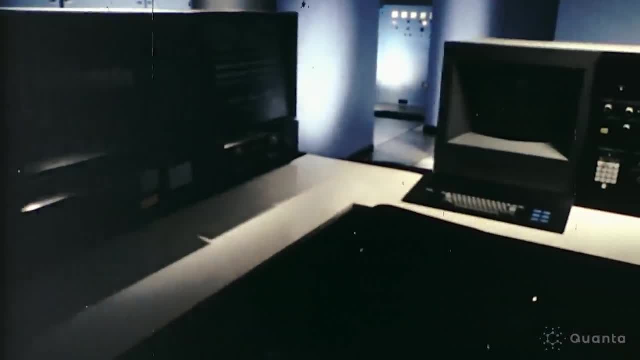 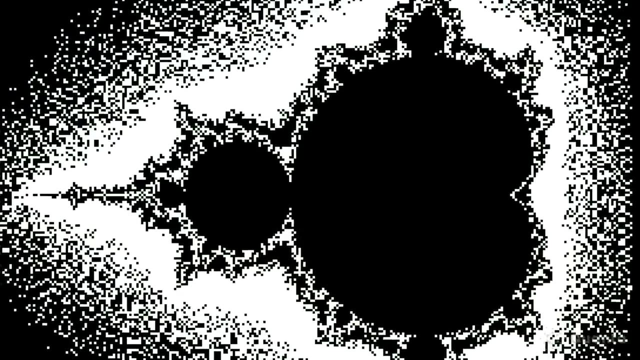 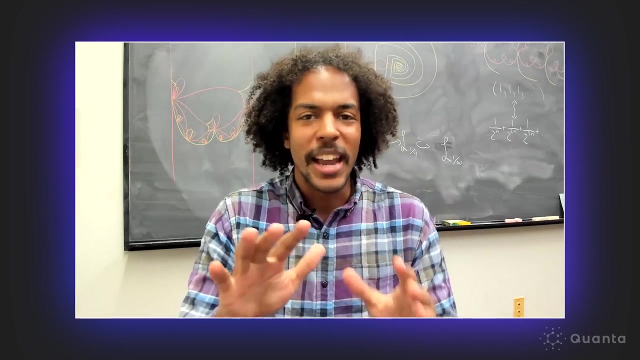 who had access to more computing power also discovered the set. This led to further explorations. These early computer graphics were crude, but the patterns revealed the presence of something far more complex, Even with fuzzy, poorly made pictures in the 80s. 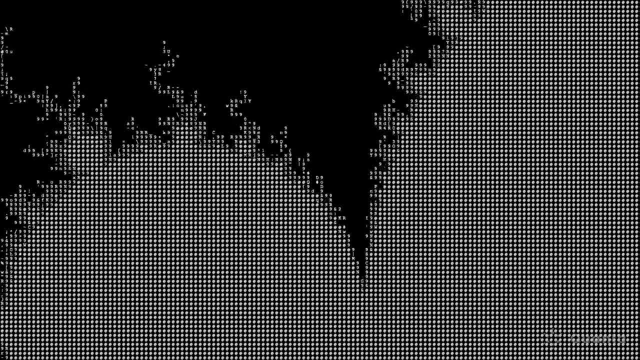 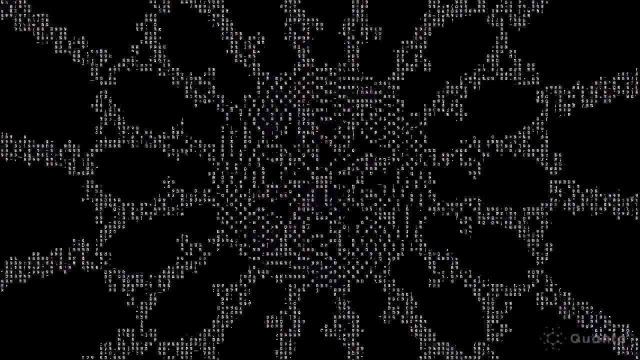 they were able to really glean a lot of interesting insight into what's going on. Mandelbrot went on to popularize his now eponymous set to the world and became known as the father of fractals. Today, mathematicians can use computers to explore the Mandelbrot set in far greater detail. 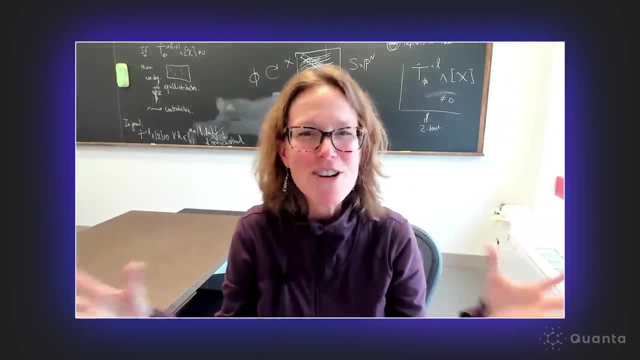 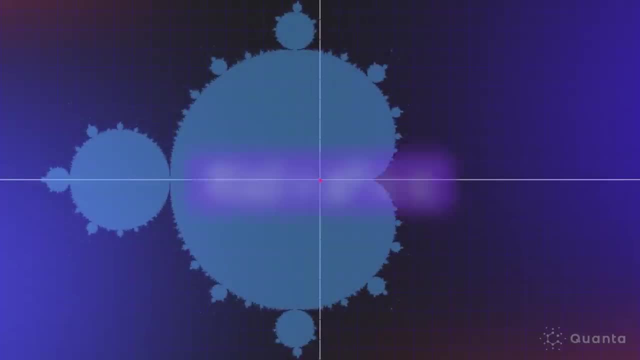 As soon as you have images, it just opens up this whole world. The Mandelbrot set is drawn in the complex plane. It's constructed by iterating the same quadratic equations used to produce Julia sets. But here things are flipped around. 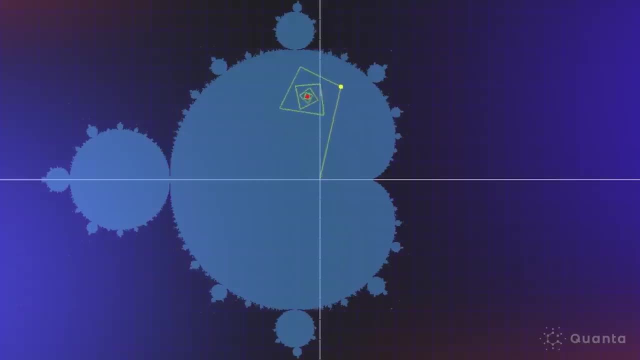 Instead of iterating all values of z for a fixed value of c, we fix the starting value of the iteration at zero and vary c Values of c. where iterations of z squared plus c stay bounded are inside the Mandelbrot set, while those that go to infinity are not. 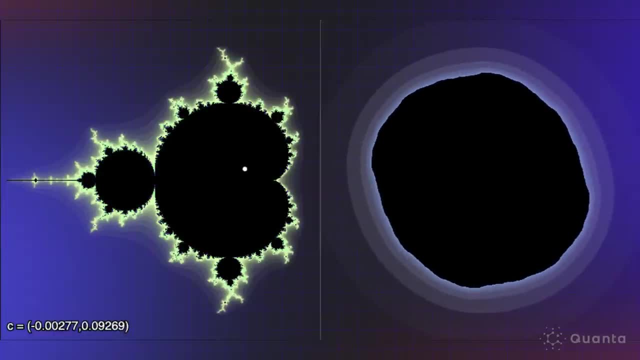 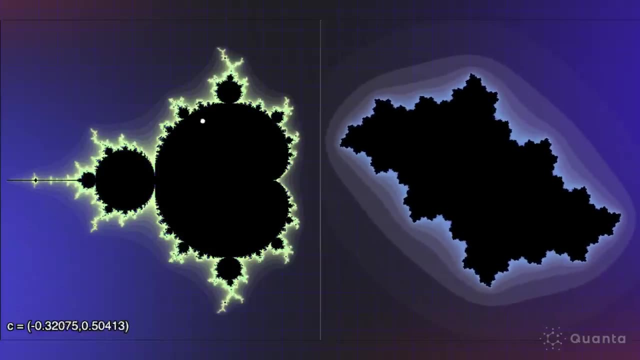 Here we can select points inside the Mandelbrot set to reveal their corresponding filled Julia sets. The Mandelbrot set acts like an atlas cataloging the different kinds of Julia sets. Values of c inside the Mandelbrot set. 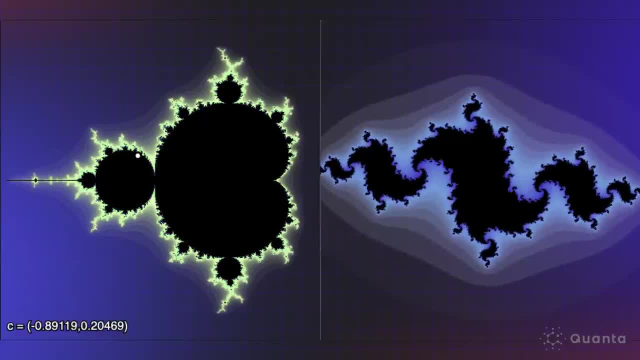 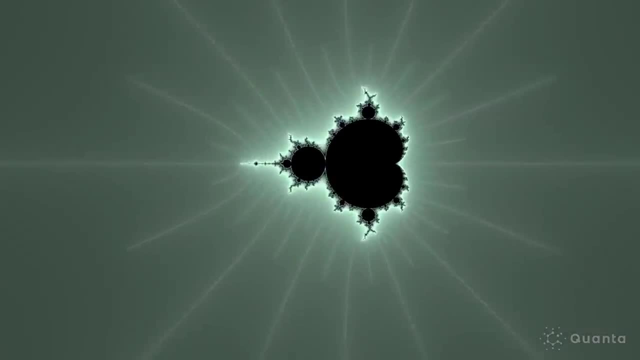 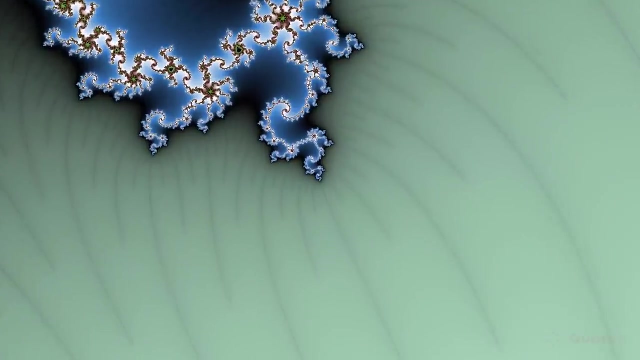 are associated with connected Julia sets, while values outside the set correspond with disconnected dust. The Mandelbrot set has many intriguing features, but its biggest mysteries lie in its complex fractal boundary. Zooming in to different boundary regions reveals some astounding features. 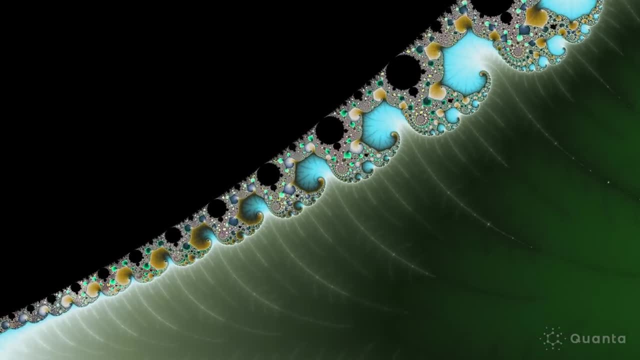 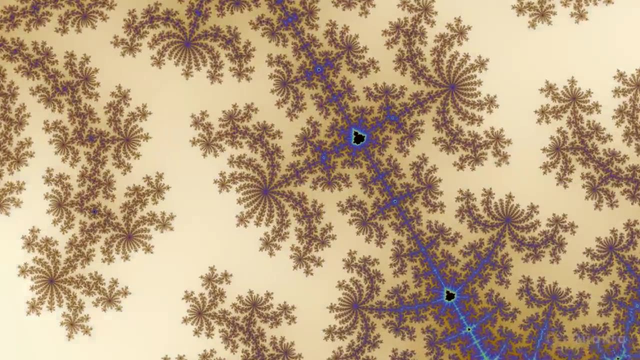 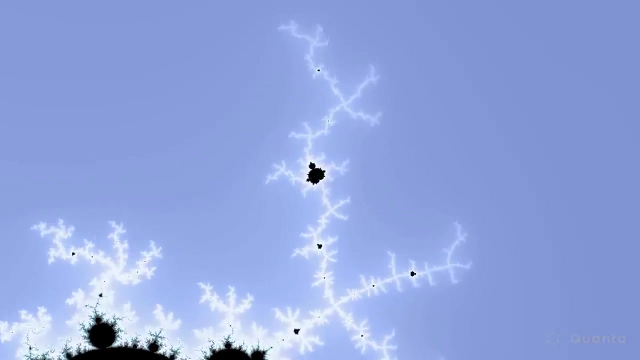 A valley of seahorses, parades of elephants and miniature versions of the set itself. So we can sort of keep finding nests- a sequence of smaller and smaller Mandelbrot sets, all one inside of the next. Here at the boundary, mathematicians are probing for answers. 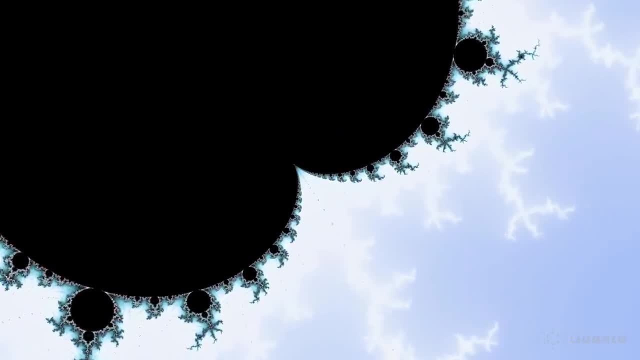 As you look at it it sort of seems like one blob, but if you really ask like, is it all connected? or maybe if I zoom in far enough, there's some separating piece. This question is central to a 40-year-old problem. 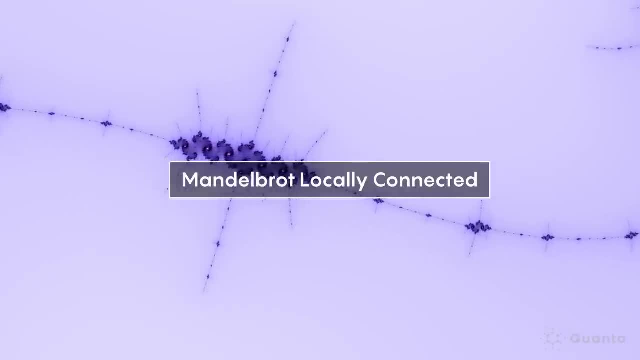 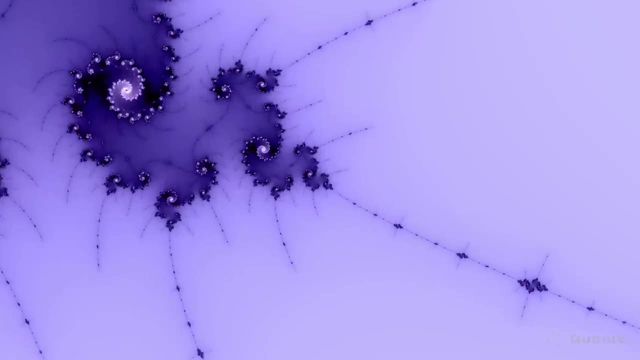 called the Mandelbrot Locally Connected Conjecture or MLC. If the set is locally connected, that means that no matter what point you choose to examine or how far you zoom in, the area will always look like one nice connected section.